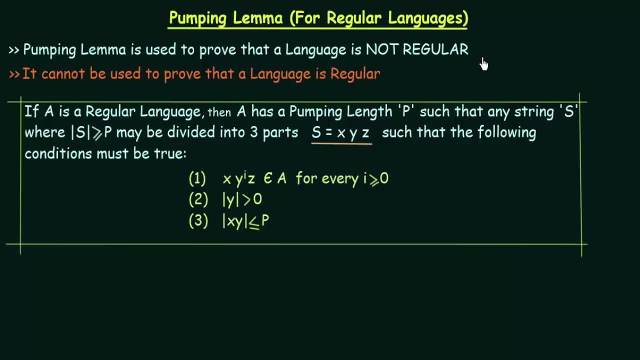 And those languages are known as non-regular languages. So how can we prove that a language is not regular? So for that we will be using this pumping lemma. So a pumping lemma is used to prove that a language is not regular. 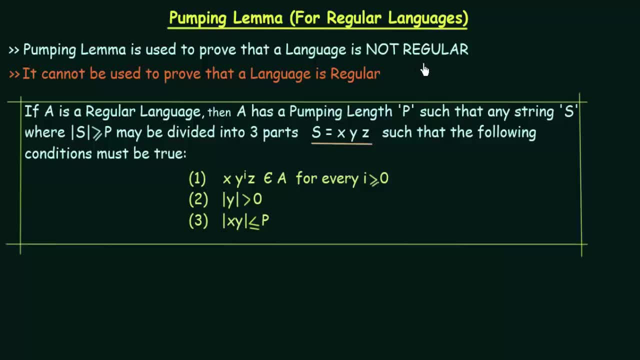 But you should keep in mind that Pumping lemma can be used to prove that a language is not regular, But it cannot be used to prove that a language is regular. It can only be used to prove that a language is not regular. Okay, so now we will see. what does the pumping lemma state and how can it be used to prove that a language is not regular? 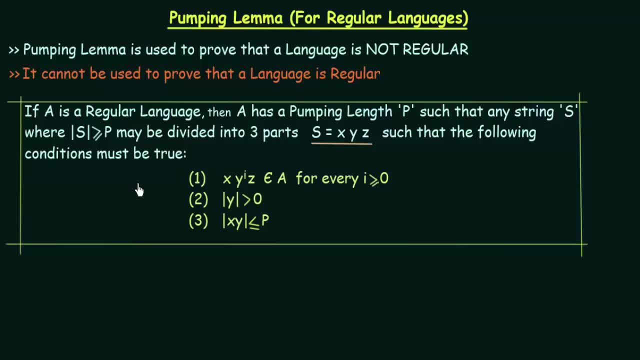 So here this is the statement of the pumping lemma given, And it says that if A is a regular language, then A has a pumping length, P, such that any string S where the length of S is greater than or equal to P may be divided into three parts: S equal to X, Y and Z- such that the following conditions must be true: 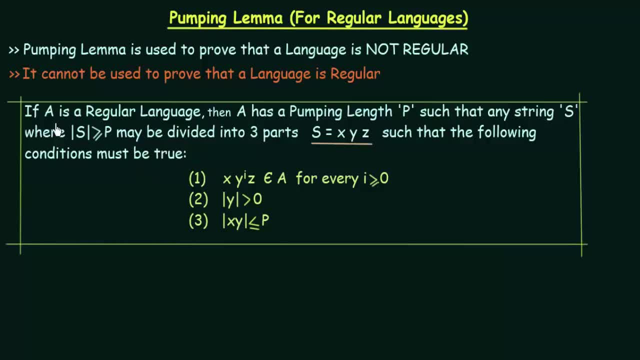 Okay, so let's try to understand this statement before we come to the conditions. So it states that if A is a regular language- suppose we have a language which is A and we assume that it is a regular language. So if A is a regular language, then A must have a pumping length P. 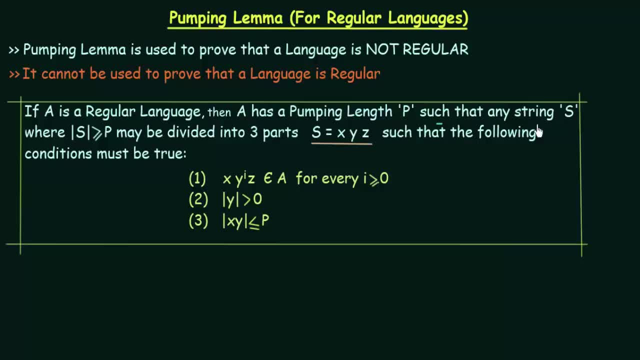 It will have a pumping length P, such that any string S where the length of S is greater than or equal to P may be divided into three parts. So if you take any string S where the length of this string S that you take out from this language A is greater than or equal to the pumping length, 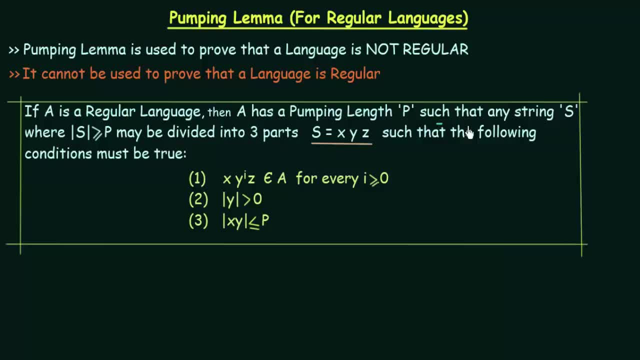 so if you take any string S where the length of this string S that you take out from this language A is greater than or equal to the pumping length. So if you take any string S where the length of this string S that you take out from this language A is greater than or equal to the pumping length, 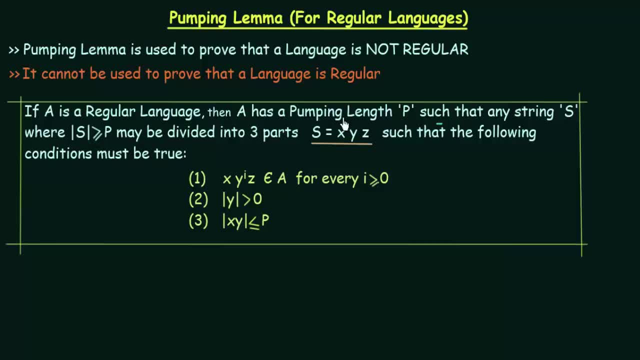 So if you take any string S where the length of this string S that you take out from this language A is greater than or equal to the pumping length, is greater than or equal to the pumping length, then this string s can be divided into three parts. 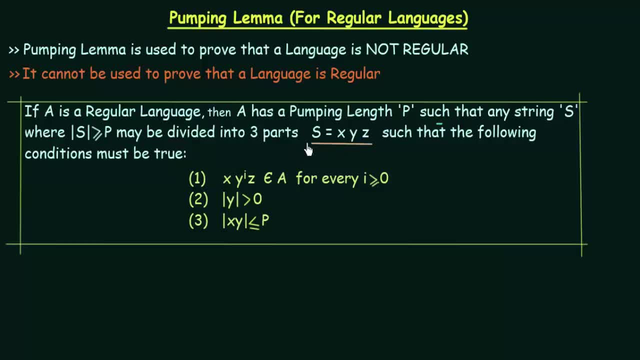 which is x, y and z. that means we take a string s which belongs to the language a and we divide that string s into three parts: x, y and z. so you have to decide how you have to divide the string into three parts, and you have to divide in such a way that the following conditions must be true: 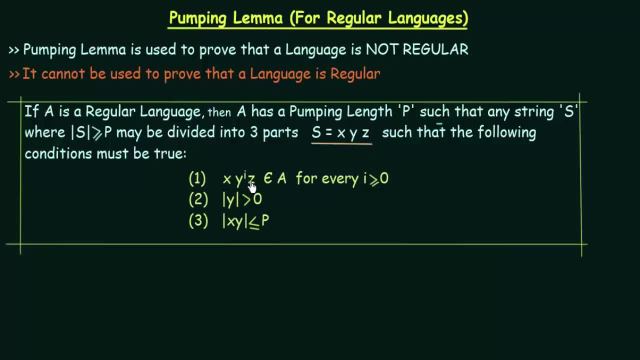 and what are the conditions x, y raised to i. z belongs to a for every i greater than or equal to zero. that means you have the string s and now you have it divided into three parts: x, y and z. and let's say that the first part x and the last part z. we keep it as it is and this middle part 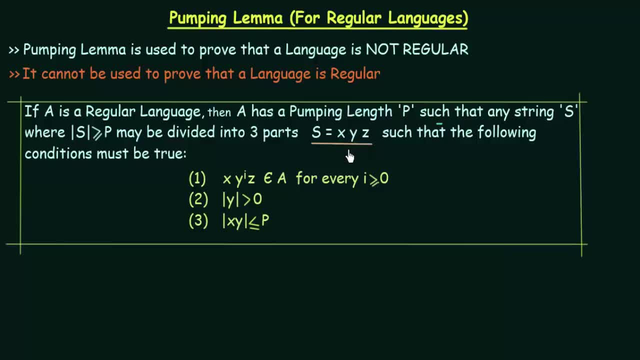 of the string, that is, y, the middle part of the string y, it may be anything. it may be some sequence of the string y, it may be anything. it may be some sequence of the string y, it may be some sequence of some kind of symbols. so this middle part y, if you increase it, if you increase. 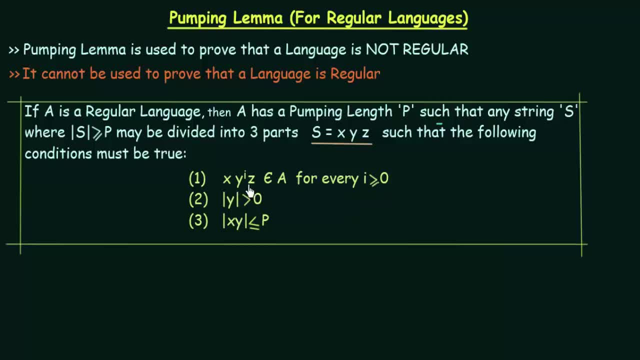 it any number of times, i greater than or equal to zero. that means, if you increase this middle part any number of times, and then the string that you obtain after increasing this y part any number of times must also belong to a. that is the language. all right. and the second condition. 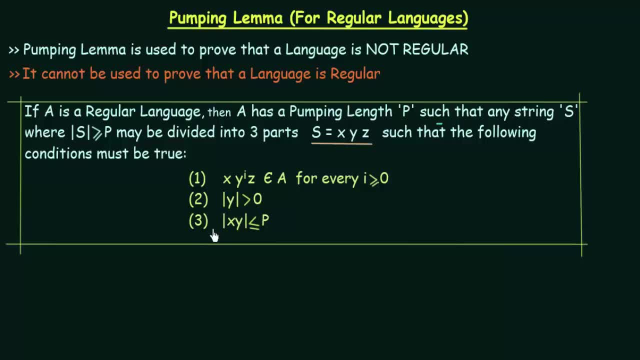 says that the length of y should be greater than zero. and the third condition says that the length of x and y together must be less than or equal to p. and what is p, which is the pumping length? so for a language to be regular, these three conditions must be true. so this is what we get from the 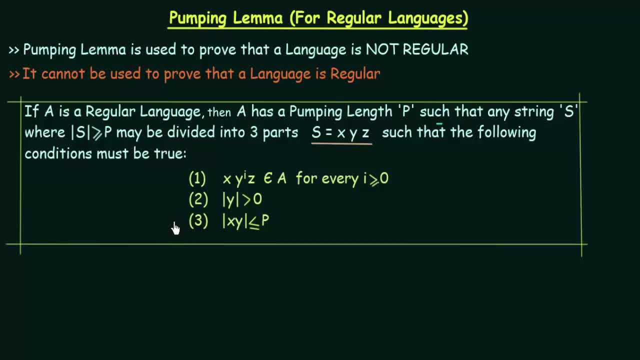 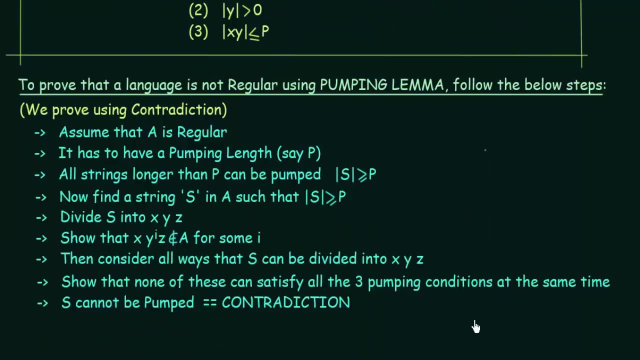 pumping lemma. and how are we going to prove that a language is not regular using this statement that we have here? let's see that, to prove that a language is not regular using pumping lemma, the below steps, and these are the steps that we are going to follow in order to prove that a 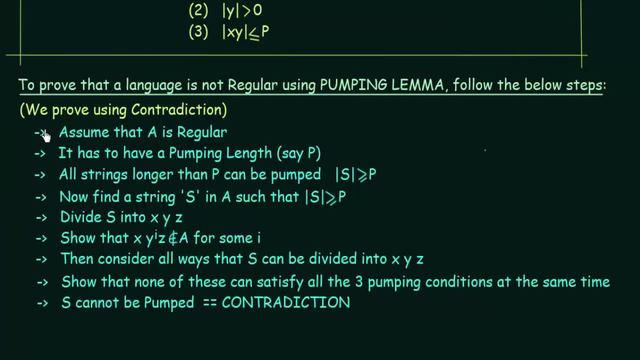 language is not regular and the proof that we are going to do is using contradiction. okay, so first of all, let's say that we have a language which we call a, and we are going to prove that a is not regular. for that what we do. since it is going to be proved by contradiction, we first assume that 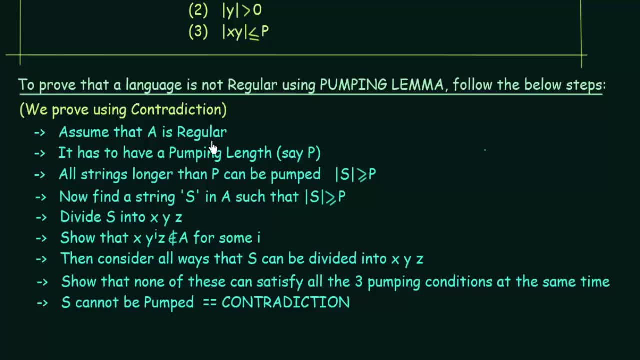 a is regular. so after we assumed that a is regular, we already read in the state behavior of pumping lemma that if a is regular then it has to have a pumping length. so let's say that it has a pumping length and we call it p. now all strings longer than p can be pumped. that means 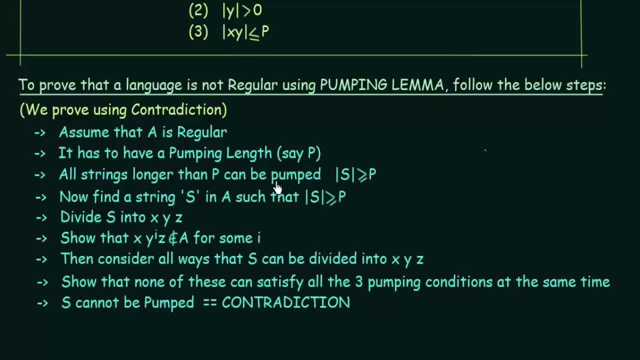 all the strings whose length is greater than or equal to p can be pumped. that we already saw in the statement of pumping lemma. now what we have to do is we have to find a string s in the language a such that the length of s is greater than or equal to p. now we are going to take a string s. 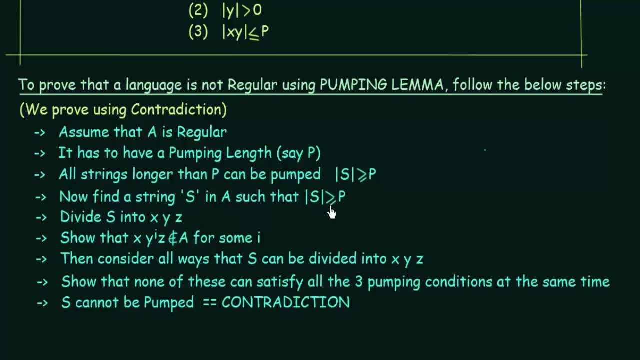 you have to choose a string s from the language a, such that its length is greater than or equal to the pumping length. after that, what you have to do is you have to divide s into three parts: x, y and z, like we already saw in the pumping lemma statement. so you divide the s that you chose. 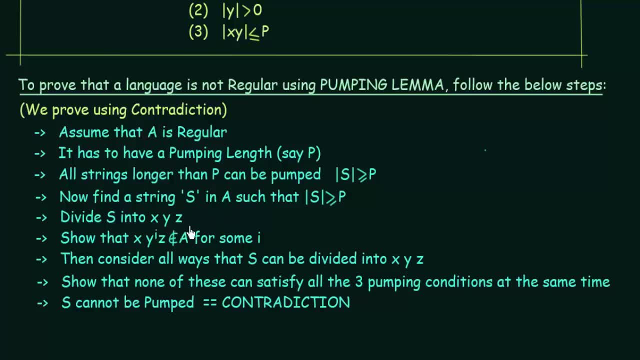 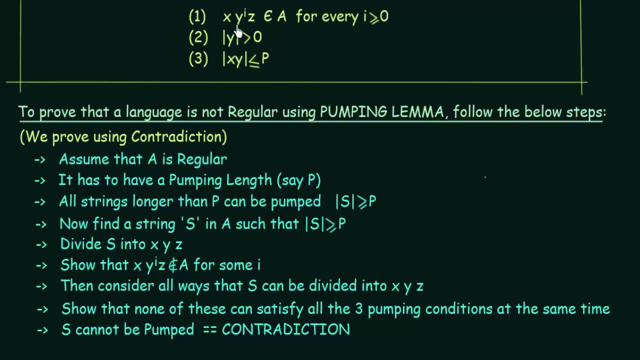 from the language a into three parts: x, y and z. now you have to show that x y raised to i, z does not belong to a for some i. so in the statement for pumping lemma we saw that if x, y raised to i, that means this middle part, y. how many time? how many? 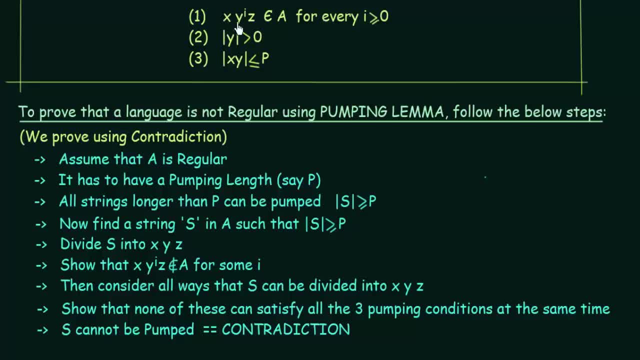 ever time you increase it, the resultant string that you obtain x- y raised to i, z must belong to a if the language is regular. so we will show that when you increase the number of this y part, the middle part and the string that you obtain as a result of x- y raised to, 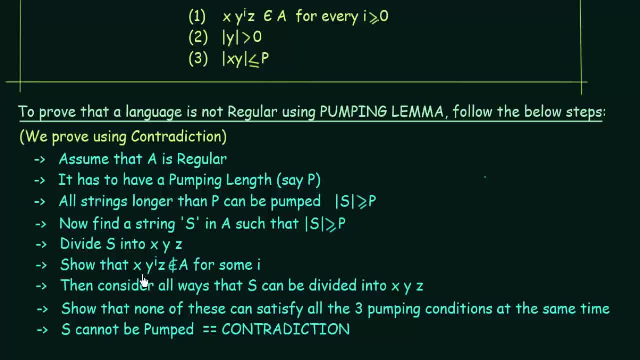 i z does not belong to a. the resulting string that you obtain does not belong to the language a. okay, and then you consider all ways that s can be divided into x, y and z. so you have to find out all the ways in which you can divide this string s into three parts: x, y and z, and you show that none of 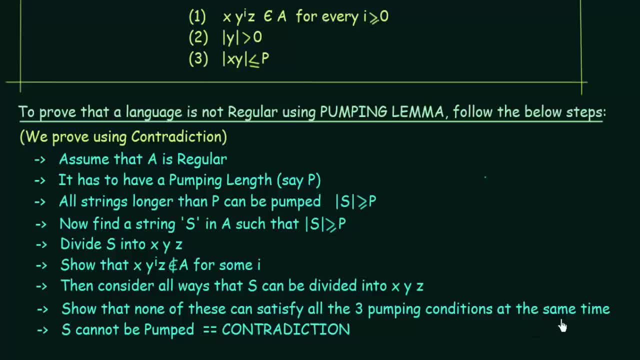 these can satisfy all the three pumping conditions at the same time. so these three conditions that we saw here, we should show that it cannot be satisfied all at the same time. so once you show that these three conditions cannot be satisfied all at the same time, then it shows that s cannot be pumped, which is a